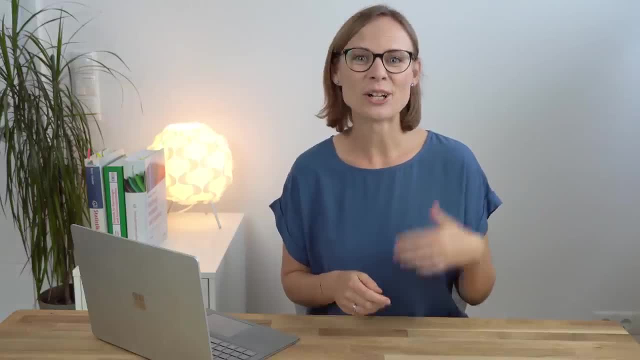 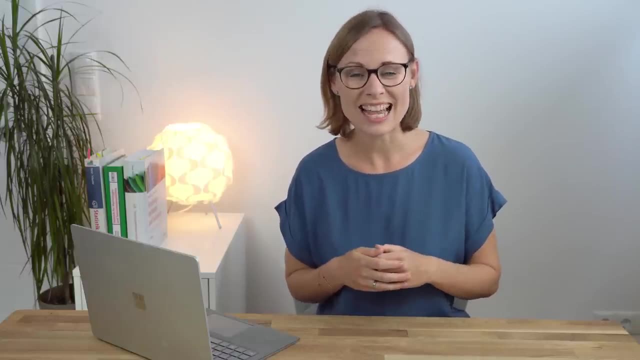 Today is about standard deviation. After this video, you will know what standard deviation is, how you can calculate it and why there are two different formulas. and, finally, what is the difference to the variance. At the end of this video, I have a tip for you. 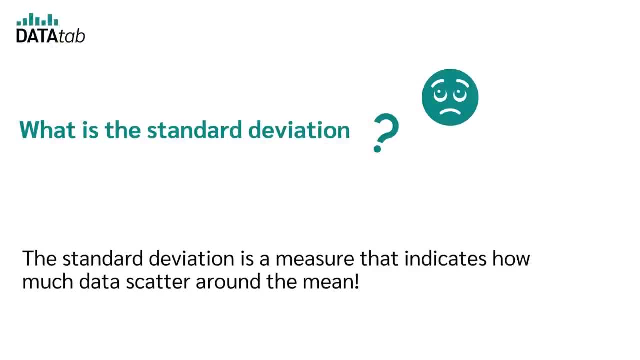 So let's get started. So what is the standard deviation? The standard deviation is a measure of how much your data scatters around the mean. So the standard deviation has something to do with the scatter of your data, for example, how different the answers of your respondents are. 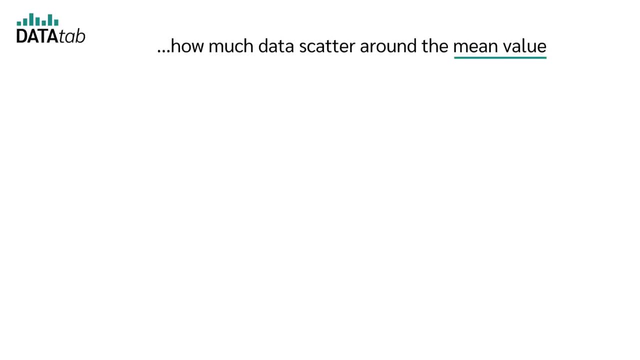 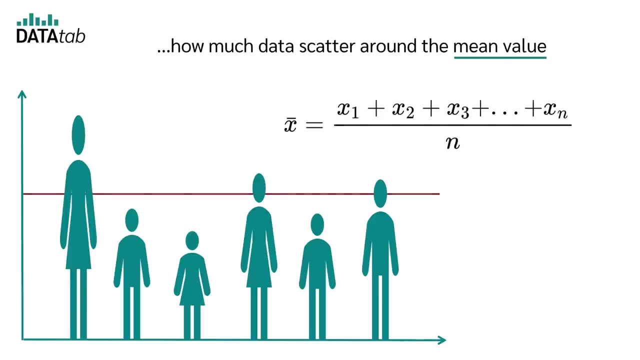 Here's an example. Let's say you measured the height of a small group of people. The standard deviation tells us how much your data scatters around the mean. So we first need to calculate the mean. You can get a mean simply by summing. 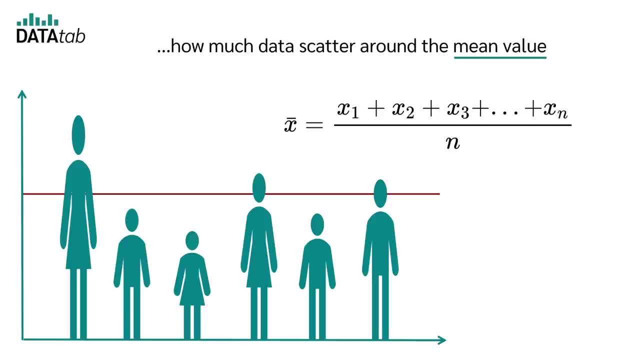 the data heights of all individuals and dividing it by the number of individuals, Let's say we get a mean value of 155 cm. Now we want to know how much each person deviates from the mean. So we look at the first person, who deviates 18 cm from the mean value. the second person deviates 8 cm from the. 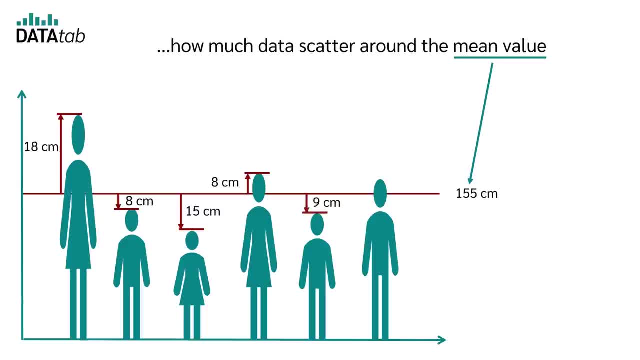 mean value, and so on. Finally, person number 6 deviates 6 cm from the mean value. So, simply said, people that are very small or very tall deviate more from the mean value. Now, of course you're not interested in the deviation of each individual person from the 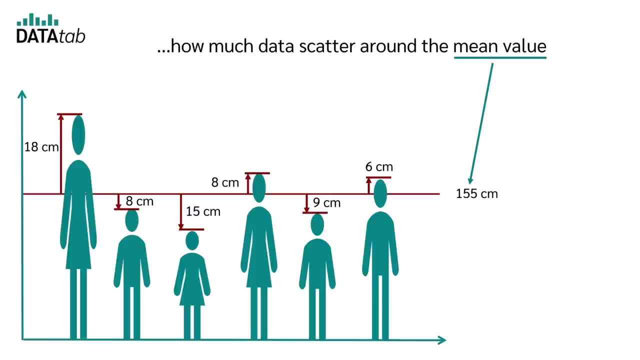 mean value, but you want to know how much the persons deviate from the mean value on average. So how much do these persons, on average, deviate from the mean value? This is what the standard deviation tells us. In our example, the average deviation from the mean value is 12.06 cm. 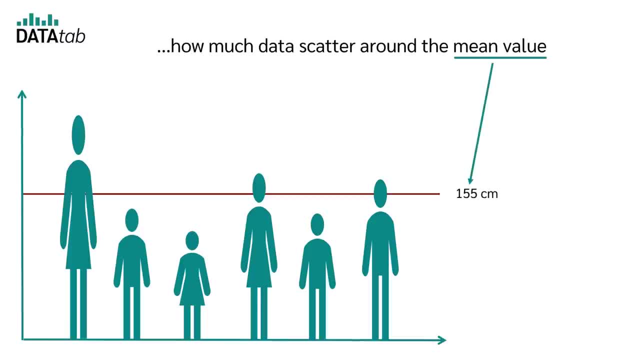 Now we want to know how much each person deviates from the mean. So we look at the first person who deviates 18 cm from the mean value. the second person deviates 8 cm from the mean value, and so on. Finally, person number 6 deviates 6 cm from the mean value. 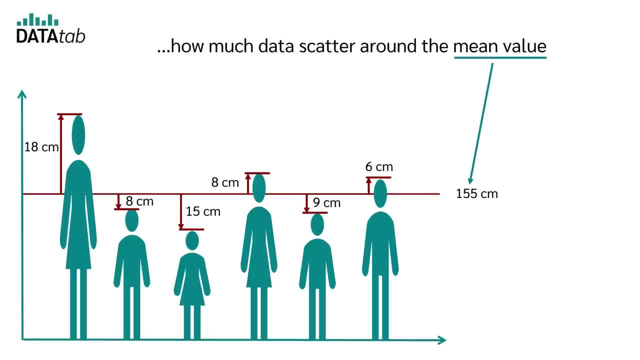 So, simply said, people that are very small or very tall deviate more from the mean value. Now, of course, you're not interested in the deviation of each individual person from the mean value, but you want to know how much the persons deviate from the mean value on average. So how much do these people deviate from the mean value? 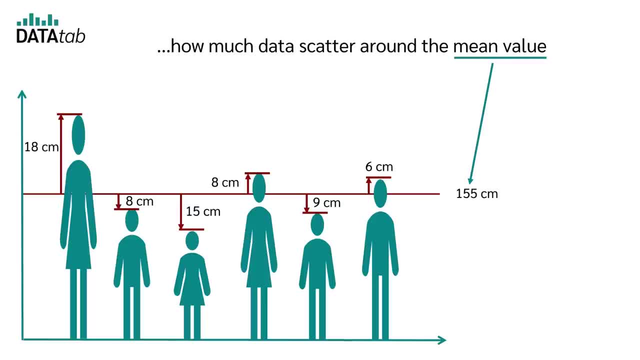 These persons, on average, deviate from the mean value. This is what the standard deviation tells us. In our example, the average deviation from the mean value is 12.06 cm. And now, of course, the next question is: how can we calculate the standard deviation? 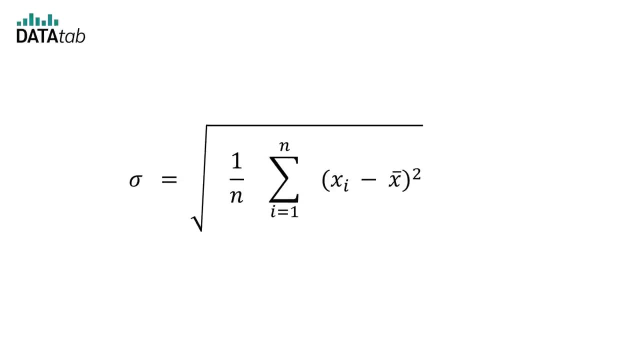 You can calculate the standard deviation with the following formula: Sigma is the standard deviation, N is the number of people who deviate from the mean value, Xi is the size of one single person And x' is the mean value of all people. 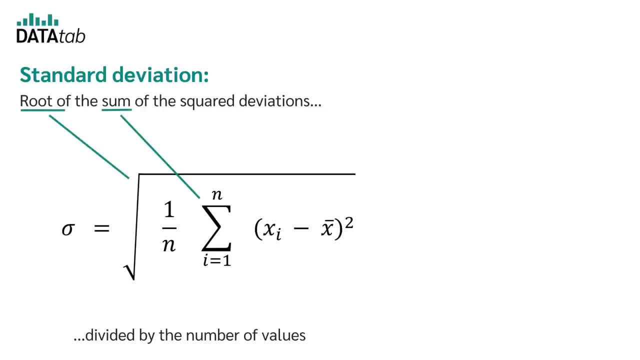 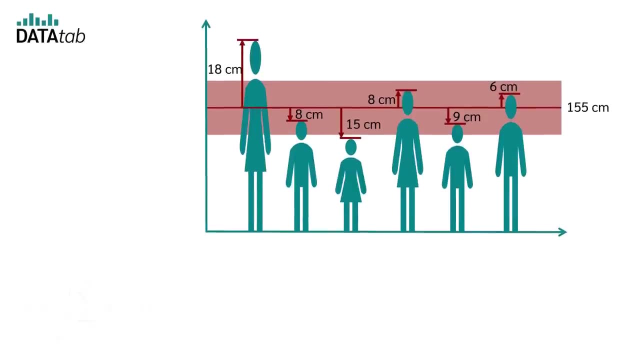 So the standard deviation is the root of the sum of squared deviations divided by the number of values. For our example, this means that we calculate the size of the first person minus the mean and square that then the size of the second person minus the mean and the. 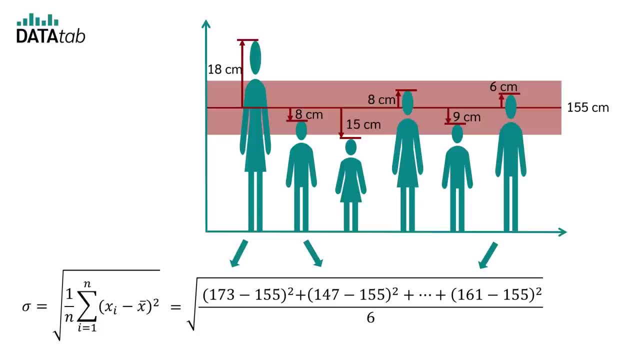 square that and so on until we arrive at the last person. Then we divide this number by the number of people, so 6, and take the root of it. The result is then 12.06 cm. So each individual person has some deviation from the mean. 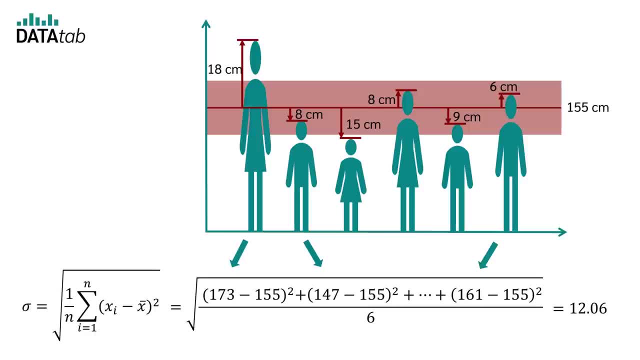 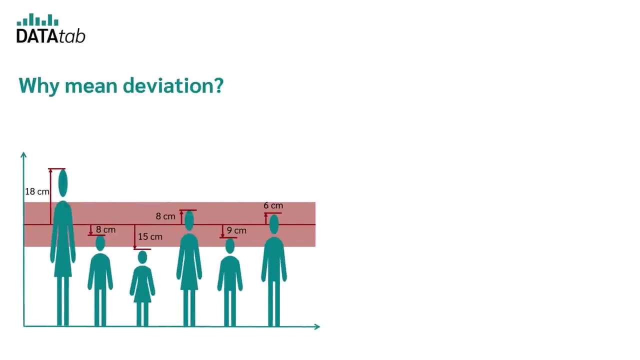 but on average the people deviate 12.06 cm from the mean, which is now our mean standard deviation. Now you might notice one thing: I always talk about the average deviation from the mean, But for the average deviation I would actually just add up all deviations. 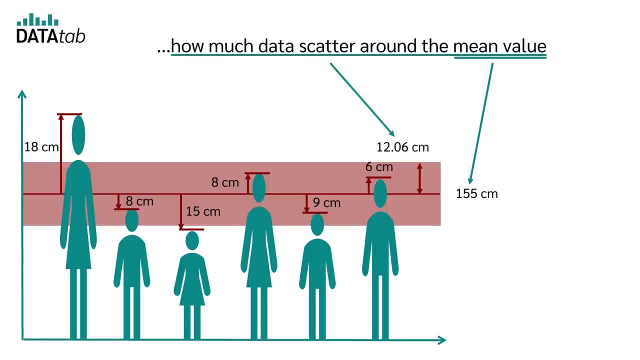 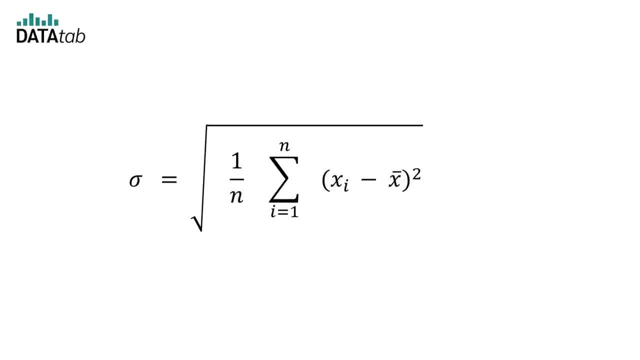 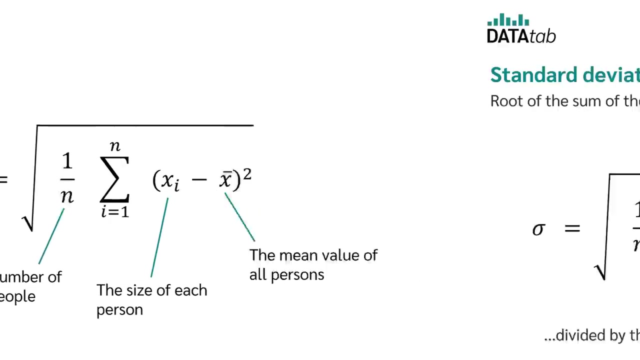 And now, of course, the next question is: how can we calculate the standard deviation? You can calculate the standard deviation with the following formula: Sigma is the standard deviation, n is the number of persons, xi is the size of one single person and x' is the mean value of all people. So the standard deviation is the root of the sum. 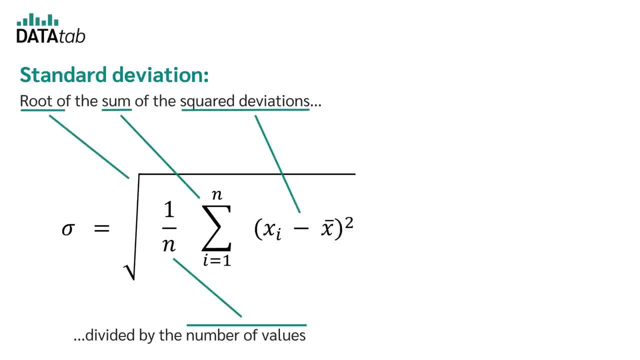 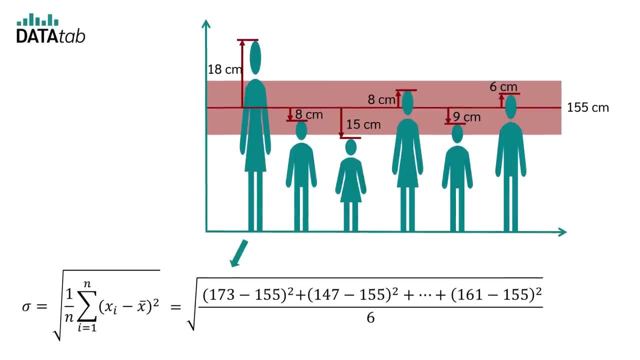 of squared deviations divided by the number of values. For our example, this means that we calculate the size of the first person minus the mean and square that, then the size of the second person minus the mean and then square that and so on until we arrive at the last person. 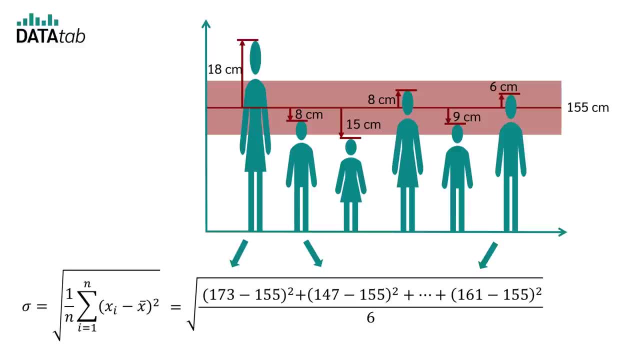 Then we divide this number by the number of people- so 6, and take the root of it. The result is then 12.06 cm. So each individual person has some deviation from the mean, but on average the people deviate 12.06 cm from the mean. 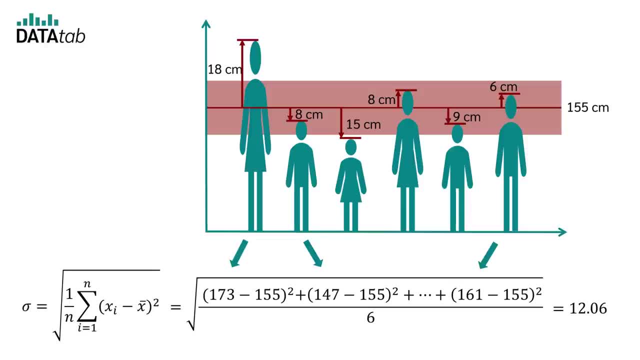 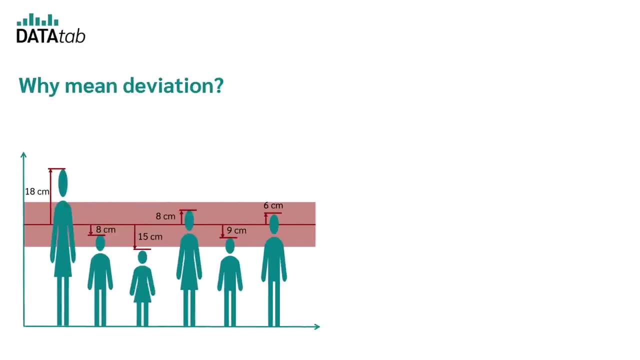 which is now our standard deviation. Now you might notice one thing: I always talk about the average deviation from the mean, But for the average deviation I would actually just add up all deviations and divide it by the number of participants, just like you calculate a mean value, right? 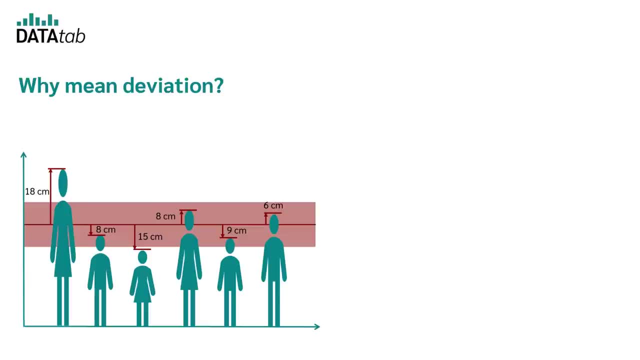 You're absolutely right, but there are different mean values. In the case of the standard deviation, it's not the arithmetic mean which is used, but the quadratic mean. If the arithmetic mean would be used, the result would be zero every time. 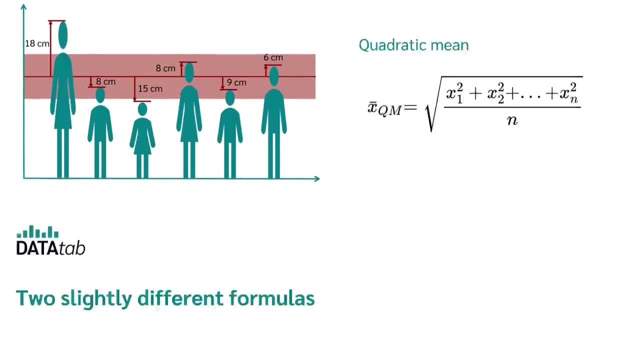 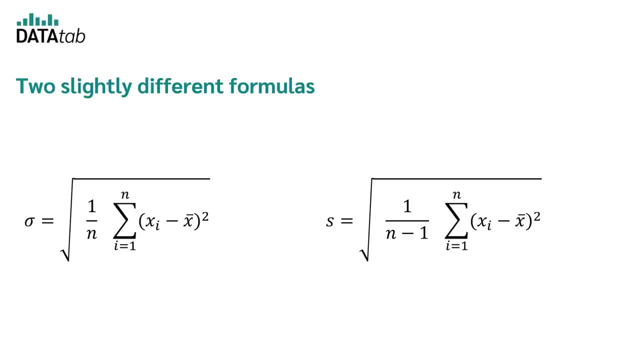 So far, so good. But now there's one more thing to consider. There are two slightly different formulas for the standard deviation. In the first formula there is a deviation by n, and in the other one there is a deviation by n-1.. Why a deviation? But why that? Why is that? What have you started with? Why is here an addition? In the first formula there is an addition by n And in the other one there is a deviation by n-1.. 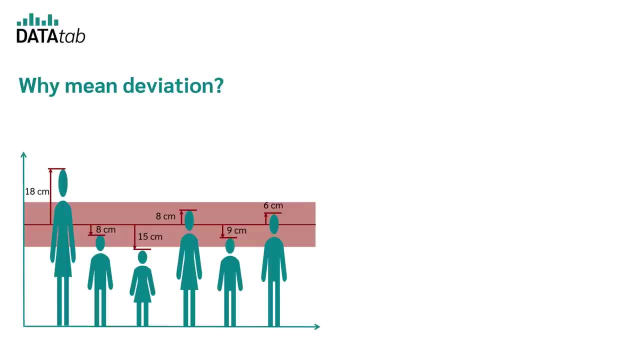 and divide it by the number of participants, just like you calculate a mean value. right, You're absolutely right. but there are different mean values. In the case of the standard deviation, it's not the arithmetic mean which is used, but the quadratic mean. If the arithmetic mean would. 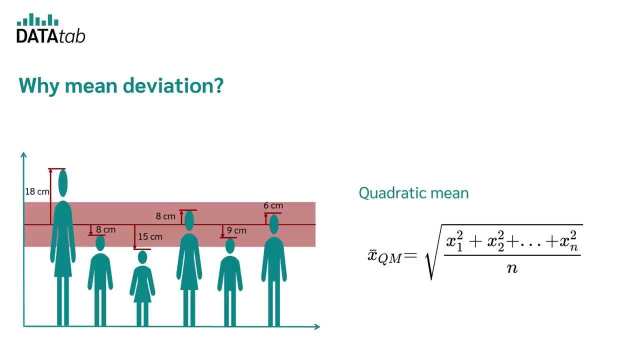 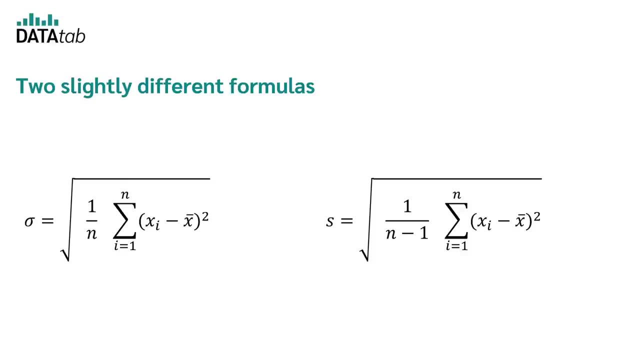 be used, the result would be zero every time. So far, so good. but now there's one more thing to consider. There are two slightly different formulas for the standard deviation. In the first formula there is a deviation by n, and in the other one there is a deviation by n minus 1.. 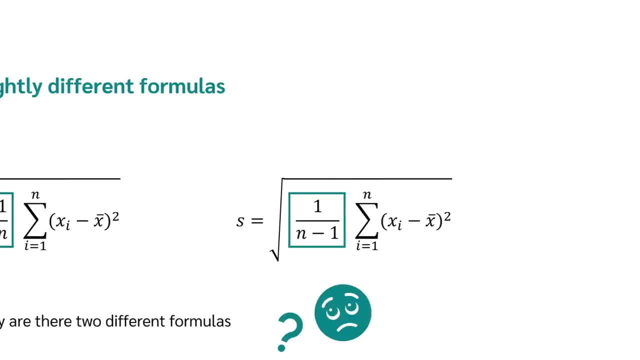 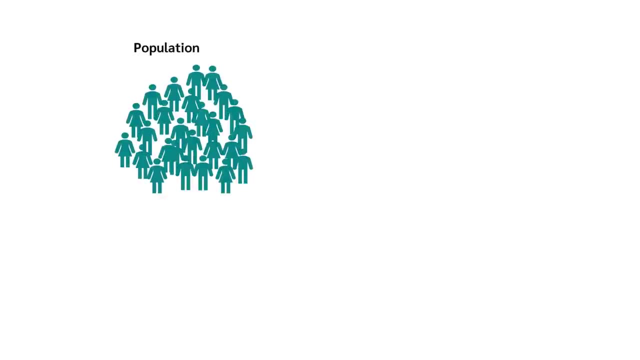 But why that? Why are there two different formulas? Usually you want to know the standard deviation of the whole population. For example, you want to know the standard deviation of height of all American professional soccer players. Now, if you had the height of all American soccer players, you would. 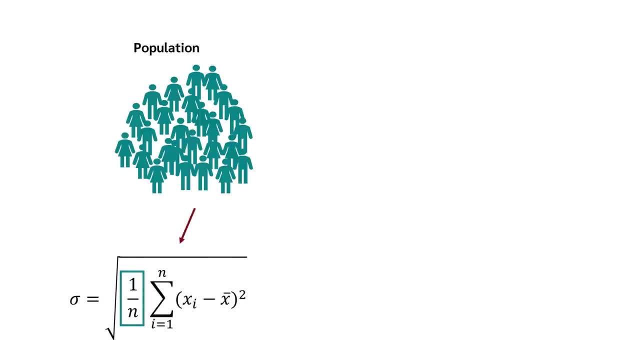 take this equation with 1 divided by n. However, it is usually not possible to investigate the entire population, So you take a sample, Then you use this sample to estimate the standard deviation of the population. In that case, you use this formula. 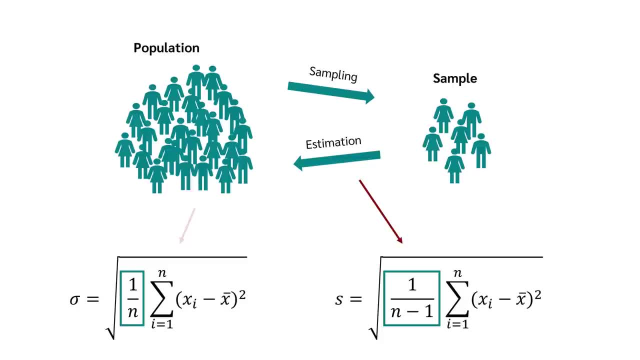 Therefore, whenever you have data of the whole population and you want to calculate the standard deviation for just this data, you use 1 divided by n. Therefore, whenever you have data of the whole population and you want to calculate the standard deviation for just this data, you use 1 divided by n. 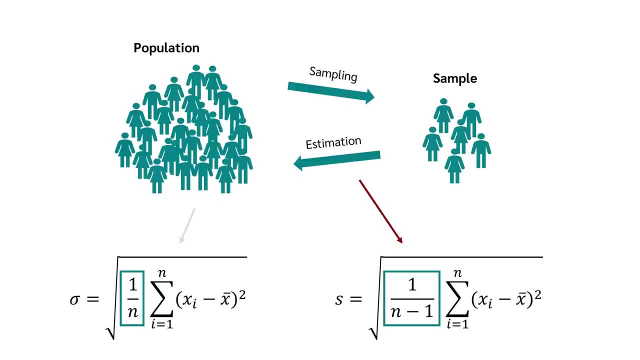 If you only have one sample and you want to estimate the standard deviation, you use n-1. So to keep it simple, if your survey doesn't cover the whole population, you always use the formula on the right side. Likewise, if you have conducted a clinical study, for example, then you also use the. In the wind. So is it true for the method you use. We would go with frequency. now, Let's so make the learning. So one betrays and then our standard deviation becomes an additional factor. So the future deviation gets different. in this situation, 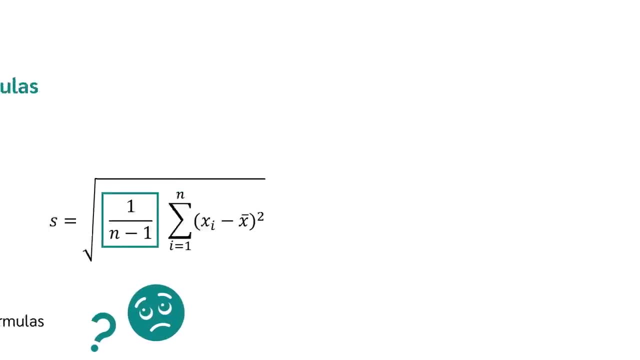 But why that? Why are there two different formulas? Usually you want to know the standard deviation of the whole population. For example, you want to know the standard deviation of height of all American professional soccer players. Now, if you had the height of all American soccer players, you would take this equation. 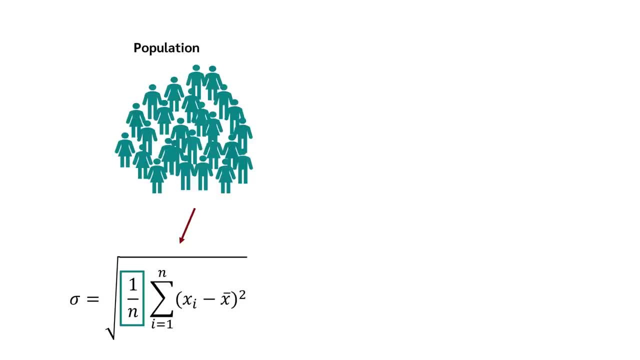 with 1 divided by n. However, it is usually not possible to investigate the entire population, so you take a sample. Then you use this sample to estimate the standard deviation of the population. In that case, you use this formula, Therefore, whenever you have data of the whole population and you want to calculate the standard. 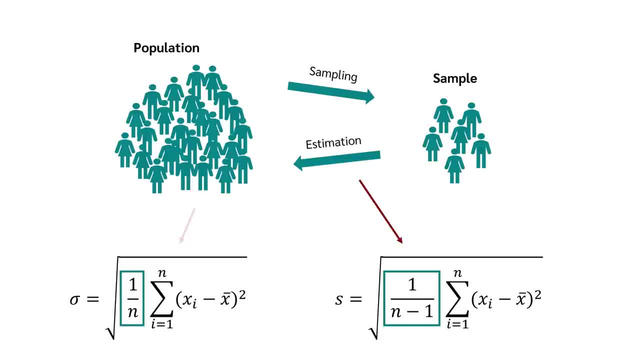 deviation. for just this data, you use 1 divided by n. Okay, Therefore, whenever you have data of the whole population and you want to calculate the standard deviation for just this data, you use 1 divided by n. If you only have one sample and you want to estimate the standard deviation, you use n-1.. 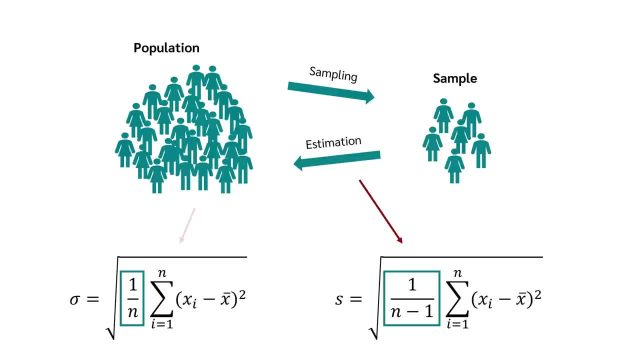 So, to keep it simple, if your survey doesn't cover the whole population, you always use the formula on the right side. Likewise, if you have conducted a clinical study, for example, then you also use the formula on the right side to infer the population. 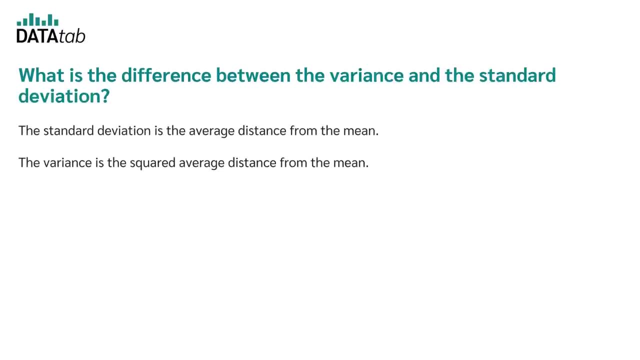 Let's look at the next question now. What is the difference between the standard deviation and the variance? As you now know, the standard deviation is the average distance from the mean. The variance now is the squared average distance from the mean. So we have one and the same formula. 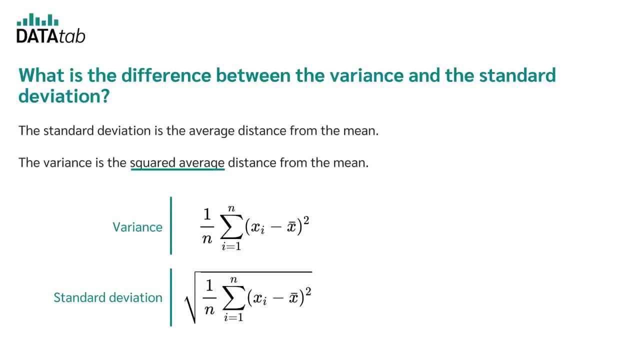 The only difference is that, in order to calculate the standard deviation, we take the root. In order to calculate the variance, we don't do that. To put it the other way around: the variance is the squared standard deviation and the standard deviation is the root of the variance. 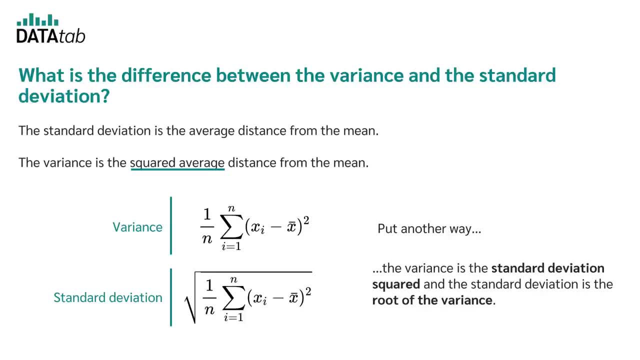 However, this squaring results in a figure which is quite difficult to interpret, Since the unit of the calculated variance does not correspond to the original data. For this reason, it is advisable to always use the standard deviation to describe a sample, as this makes interpretation a lot easier for you. 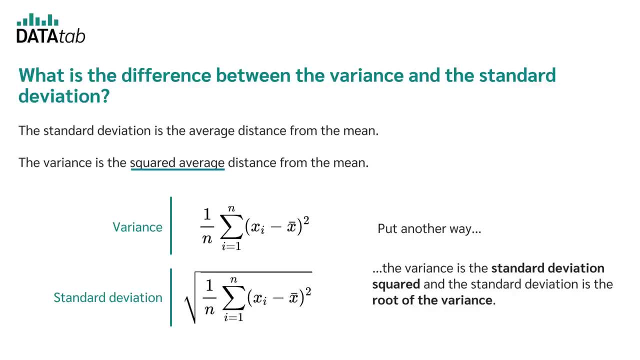 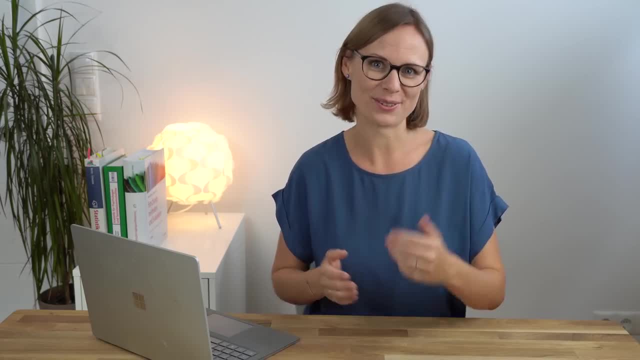 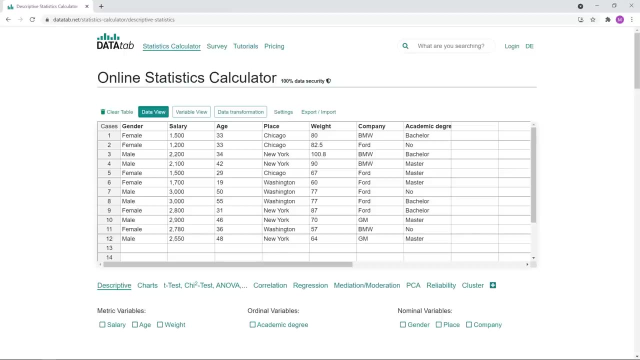 The standard deviation is always in the same unit as the original data. In our example, this would be centimeters. And finally, as promised, I have a tip for you. If you want to calculate the standard deviation, you can easily do it online with Datatab. 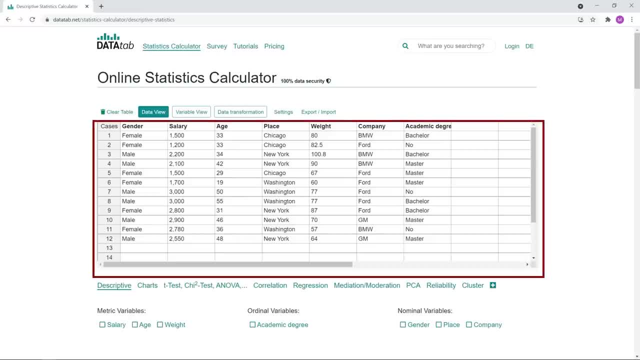 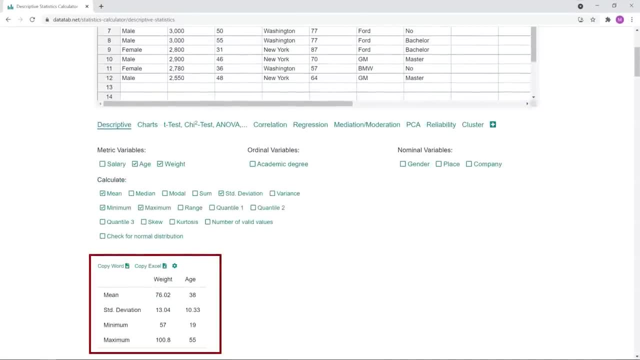 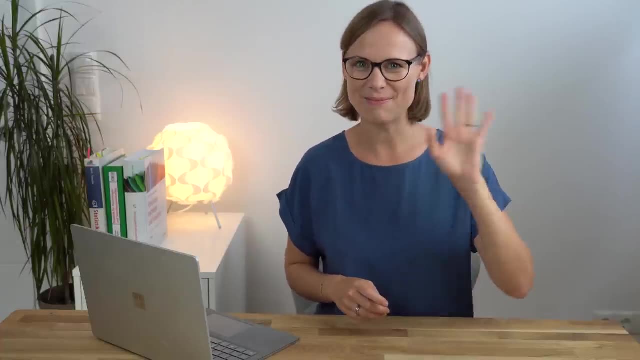 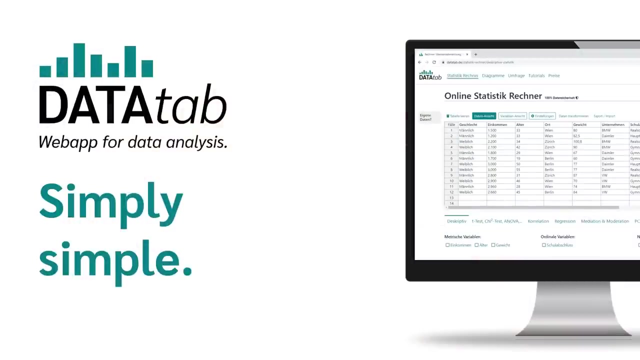 Just visit datatabnet, copy your data into the table, select the variable you want to calculate and afterwards you will get the standard deviation in a very easy way. I hope you enjoyed the video and see you next time. Bye, bye, wwwdatatabnet. 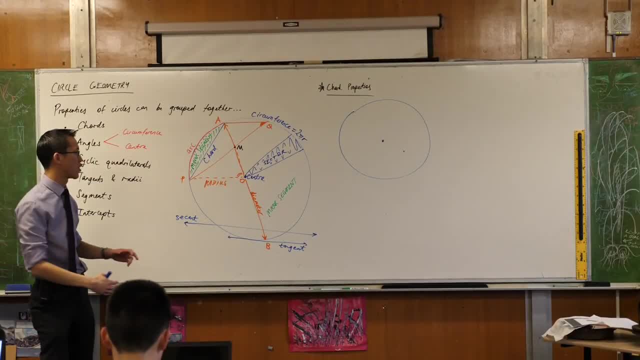 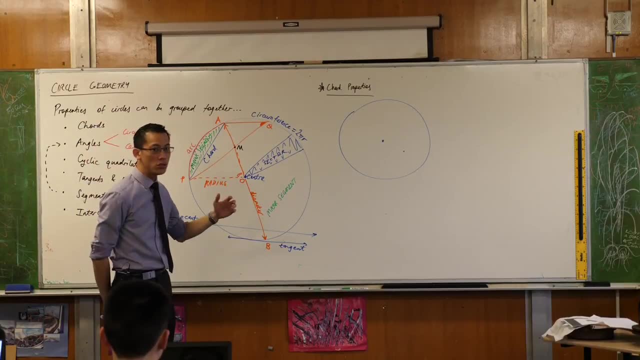 You've got a circle- any circle. These ones can be a bit smaller because we're not going to put such a huge number of things on them. okay, Draw a circle, any circle, and then what I'd like you to do is: onto your circle, I'd like you to draw. 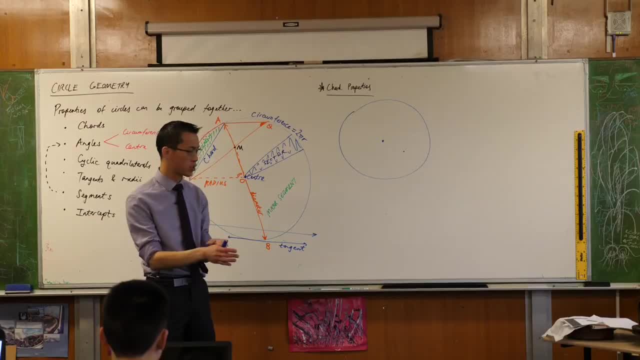 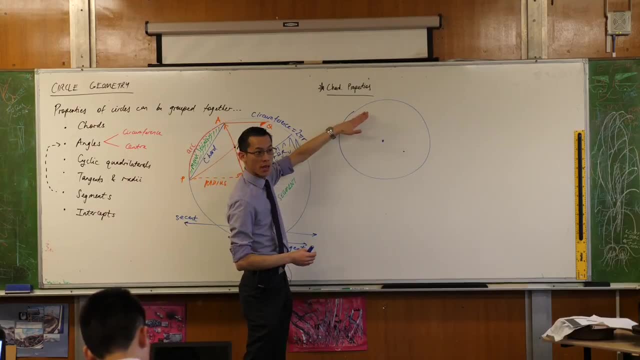 a pair of cords. But here's what I want you to do with these cords specifically. Can you just make the cords the same length? Make the cords the same length, So maybe they're both going to be two centimeter cords, but in different spots. 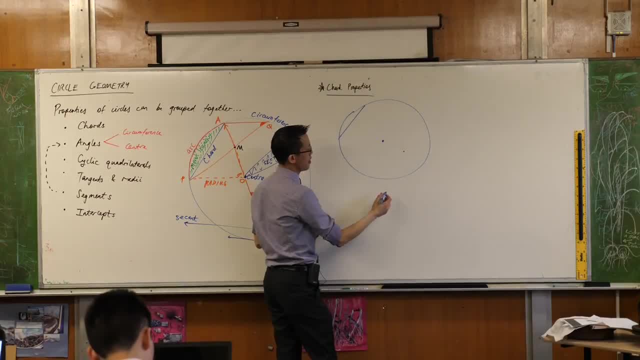 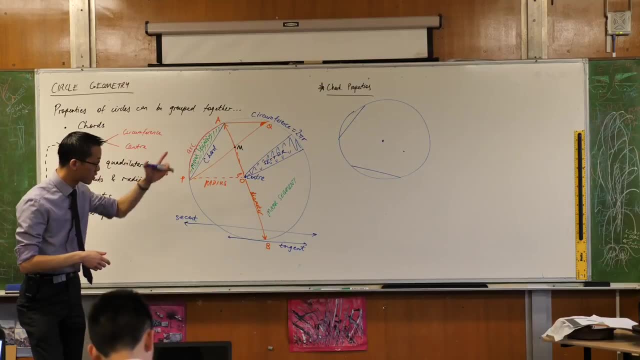 Maybe something like over here and over here. okay, You can make them short, You can make them long, You can make them overlap, You can make them not touch each other, like mine don't, Once you've made them the same length, and it'd be really.